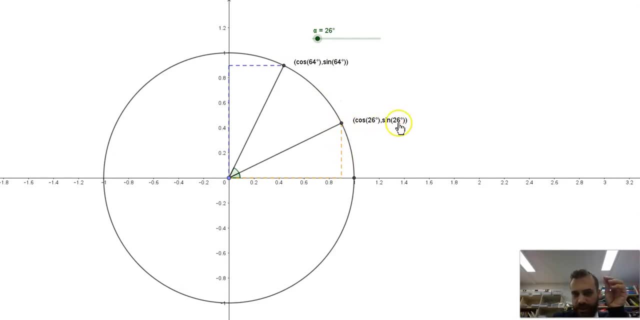 So we can see that this is the x-coordinate of this dot. this is equal to this length here, which is this bit here. So, in other words, cos 64 is equal to sine 26 and similarly, this length here, which represents cos 26, is equal to this line here, which is the y-coordinate of this dot, which is: 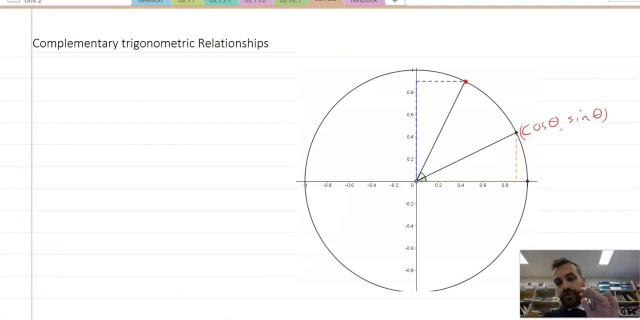 sine 64.. So now to generalize this, what I'm saying is that if this line is the y-coordinate of this dot angle here is theta and this angle here is theta, then this angle here let's draw a nice big one- here is pi minus theta, sorry, pi on 2 minus theta, pi on 2, 90 degrees minus theta, because 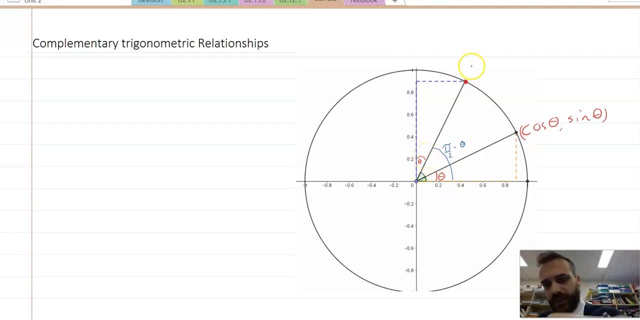 that's there Now. the coordinates of this dot can be described in two ways. We can say that the coordinates of this dot are cos pi on 2 minus theta, sine pi on 2 minus theta. but we could also say that the coordinates of that dot are equal to. we can move this y. 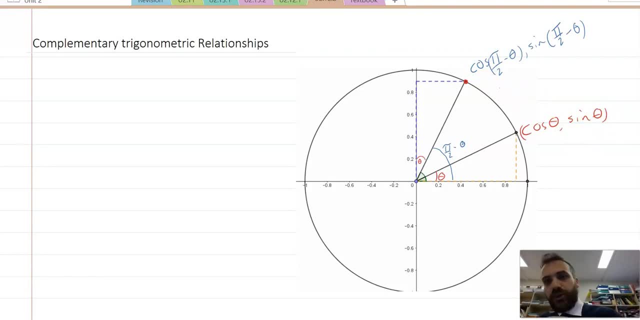 coordinate over here, so we can say that the coordinates of the dot could also be sine theta, cos theta We're through. theta is the angle between the y-axis and this point here. Now the upshot of this is really straightforward: We get this complementary relationship So sine pi on 2 minus theta. 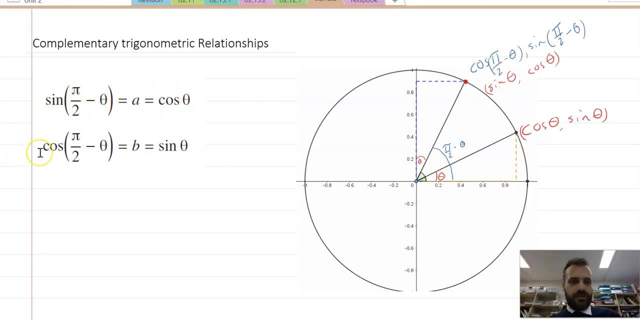 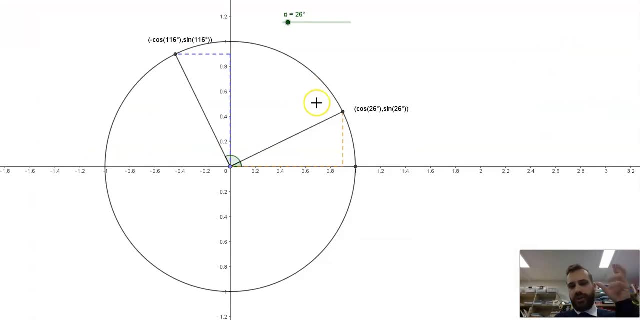 is equal to cos theta And cos pi on 2 minus theta is equal to sine theta. We don't need to worry about these little a's and b's here. Hopefully you can appreciate that this occurs in all four quadrants. So here we have the angle theta, in this case cos 26.. And here we have a larger angle. 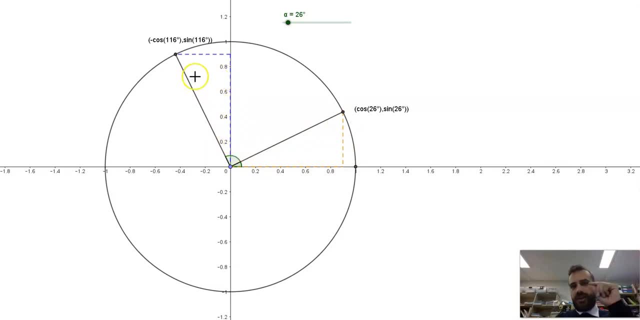 cos 90 degrees plus 26,, which is 116 degrees. Now, in this case, we still get this nice line here that's equal to this line here. We also get this line here, which is equal to this line here. Now, the only difference is that this negative here, right, Because we're in. 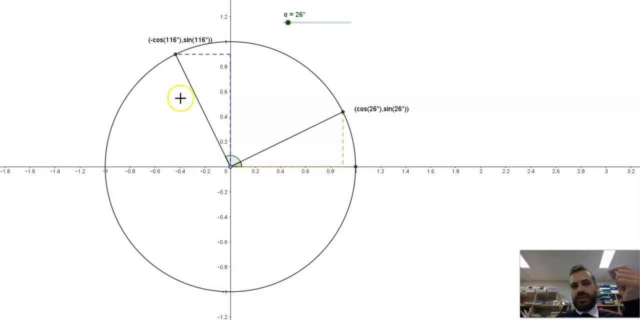 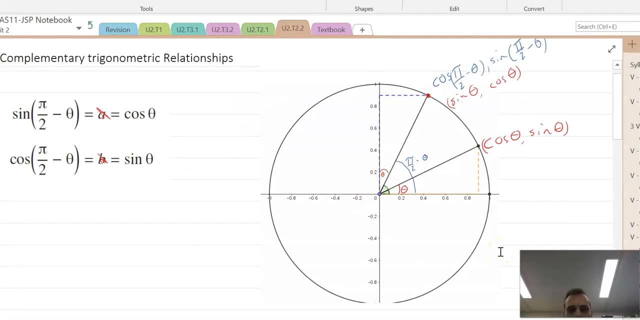 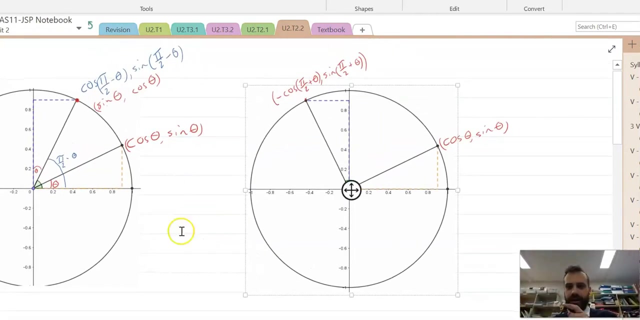 in the second quadrant. so x coordinates are going to be negative. So we have this relationship. So this was our first quadrant relationship. Now, if I move over here, we get our second quadrant relationship here where we can say that cos theta sine theta here. 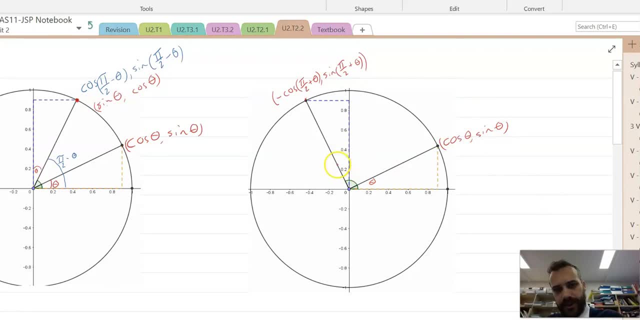 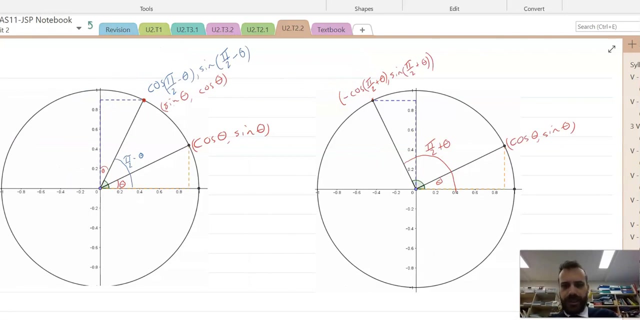 where theta is. this angle here, Now this angle all the way around here, is pi on 2 plus theta, And that means that that's going to be equal to negative cos, pi on 2 plus theta, sine pi on 2 plus theta. But we can simplify both of those in the same way that we simplified it here, to just be. 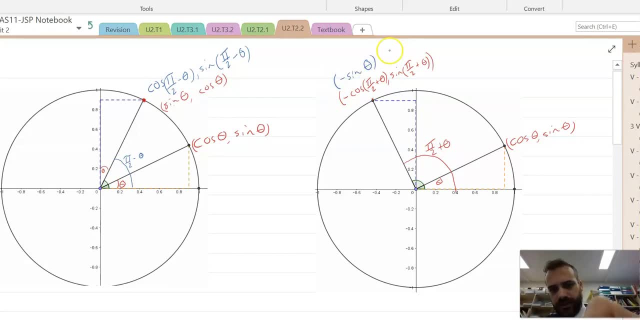 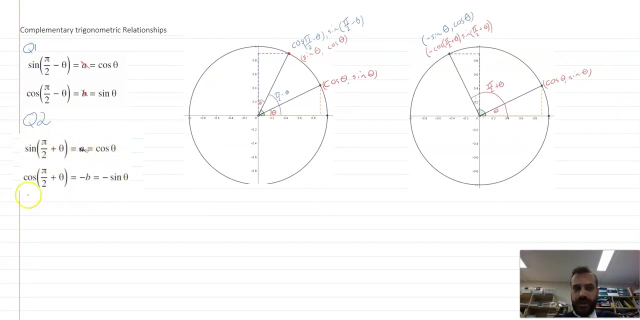 negative sine theta, cos theta Because the cos theta is this, sorry, this length here, And so that cos theta represents that length there And the negative sine theta represents that length there. That leads us to our second quadrant relationships of sine pi on 2 plus theta being equal to cos theta and cos pi on 2 plus theta. 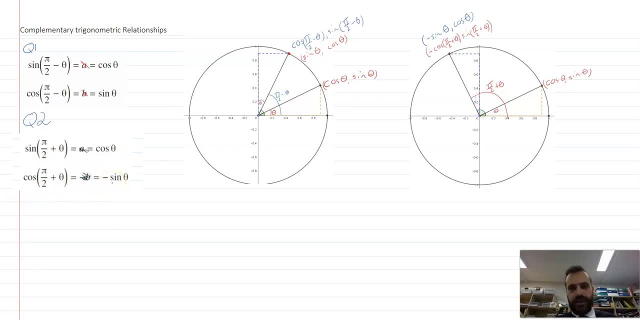 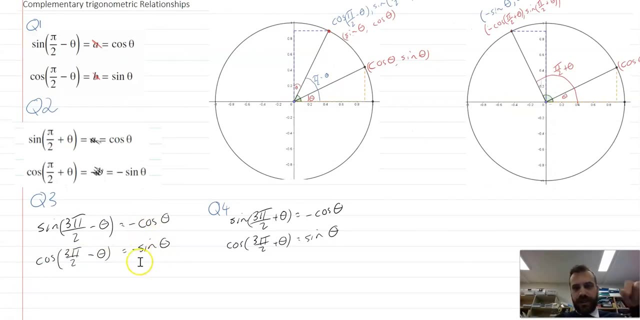 being equal to negative sine theta. Now of course there are third quadrant and fourth quadrant relationships as well. Q3, they're both going to be negative. But in Q4, here sine 3 pi on 2 plus theta, that represents the y coordinate And the y coordinate. 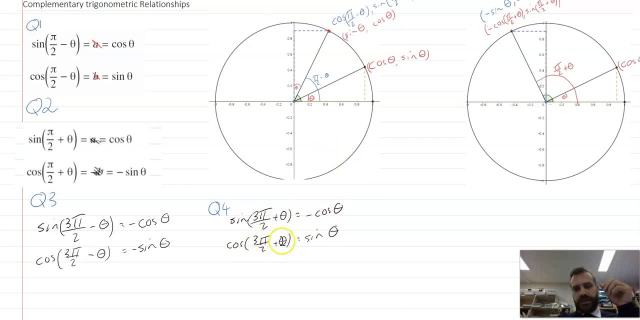 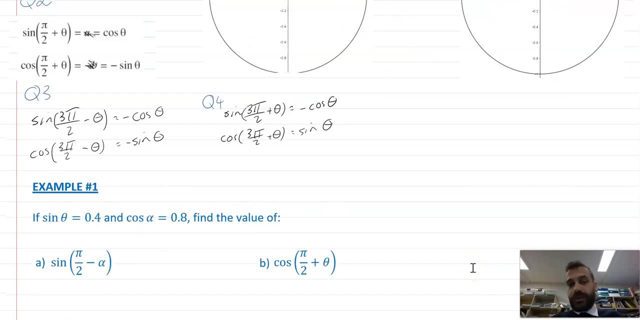 it's going to be negative in Q4.. And cos 3, pi on 2 plus theta, that represents the x coordinate, and the x coordinate is going to be positive. Now what can we do with this? Questions that look a little bit like this. But if we know that the value of sine theta is 0.4 and the value of cos, 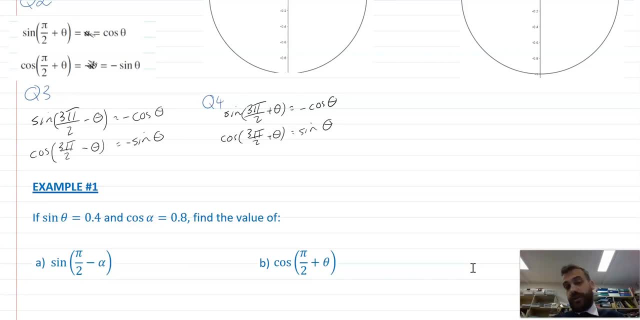 alpha is 0.8, we can find the value of sine pi on 2 minus alpha, Because we know that sine pi on 2 minus alpha is equal to cos alpha And we know that cos alpha is 0.8.. Now this one here: cos pi on 2 plus theta. Now we know that. 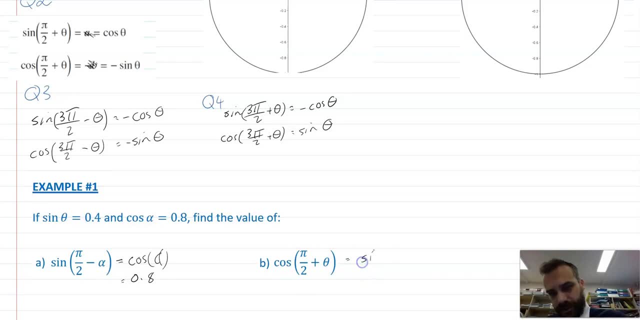 cos pi on 2 plus theta is going to be equal to sine theta. But you might just want to draw yourself a little circle here and say: right, what am I doing? Cos pi on 2 plus theta. I'm doing this angle here, which is the same as this angle here, And I'm going to draw a little circle here And